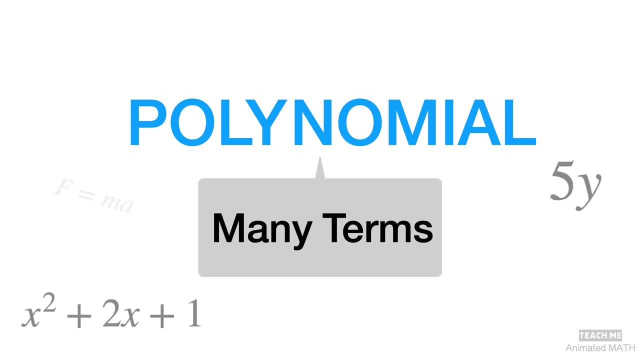 And that is why polynomials look very different from each other, And to some of us they might look quite intimidating. Oh, but I'll tell you a secret: Each polynomial is like a psychic power: Psy, Psyduck, Yep, you heard that right. 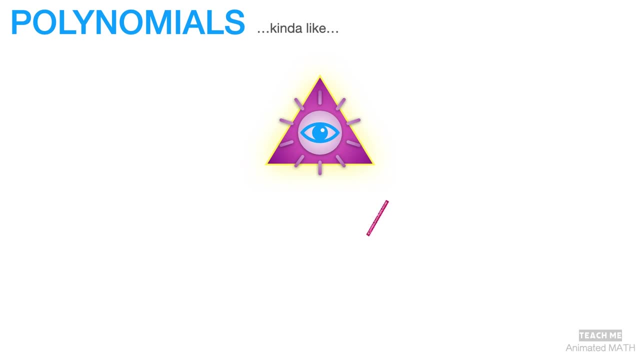 Polynomials are like psychic power-ups that grant you clairvoyance or the power of foresight. Some people use this power every day without realizing it, while others do it more consciously. A very basic example of it is when you buy something in the supermarket. 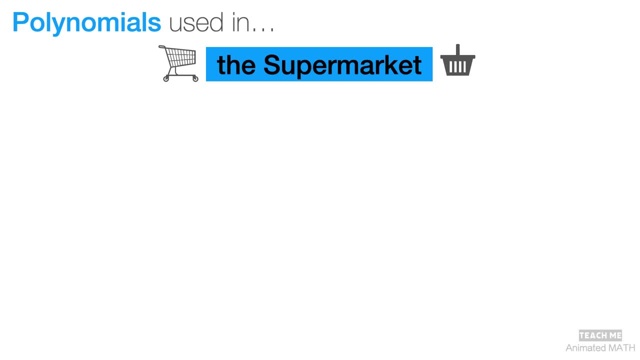 You might want to know how much your baking ingredients might cost, For example, four kilograms of flour, three dozen eggs and two liters of milk. Before you even check the prices, you might unconsciously construct this equation in your head And, whatever the price of each ingredient is, you'll be able to predict the total cost. 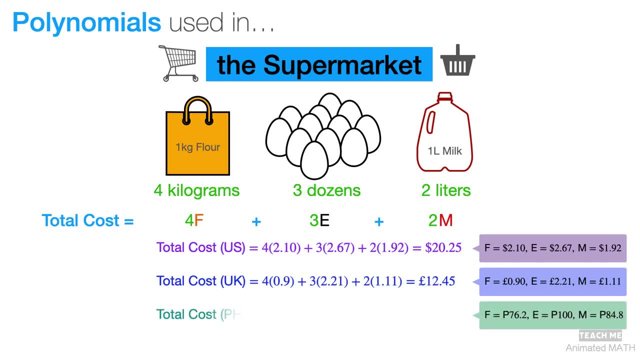 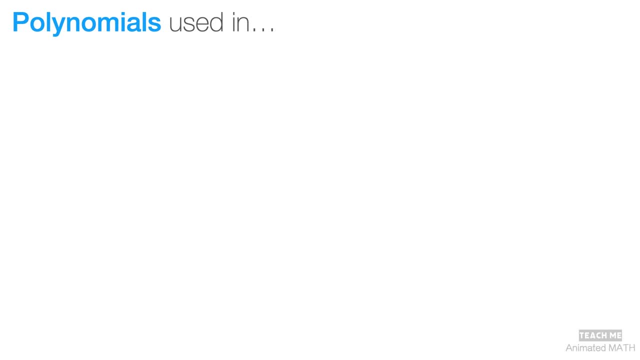 The total cost with the help of your psychic power or the polynomial equation. And, believe it or not, it can also be used in the area of love. What A book called The Five Love Languages was authored by Gary Chapman And in December 2010, 10,000 people took his online quiz, which resulted in this: 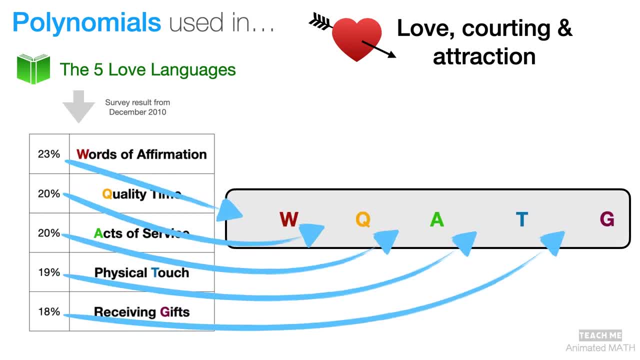 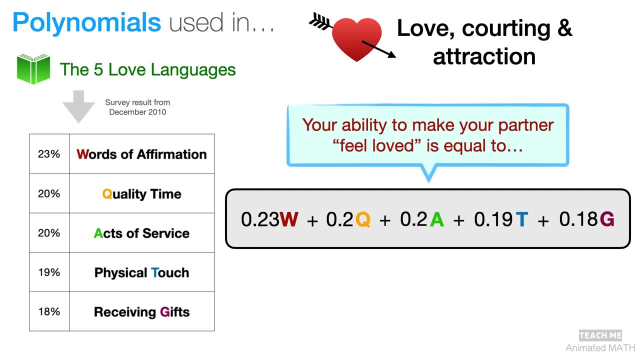 That result can be converted into this formula. And, yes, what you're looking at right now is a polynomial. It says that, in general, your ability to make your partner feel loved is determined by the values of your W, Q, A, T and G and which love language they respond to. 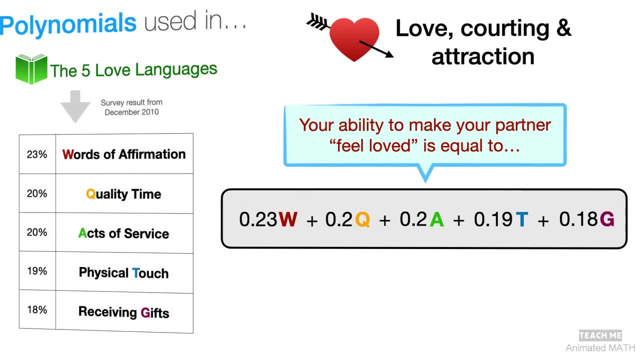 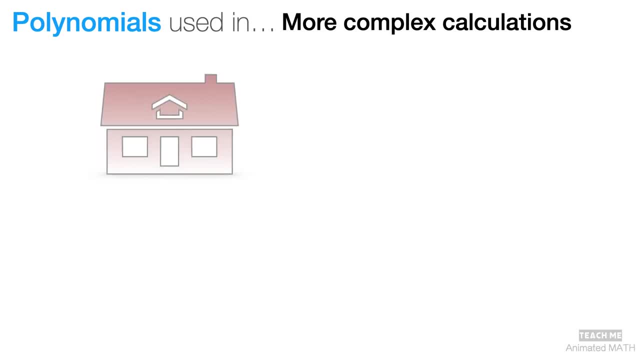 Interesting right. Polynomials are also used in more complex calculations. For example, an engineer designing a house so that the roof doesn't collapse from a heavy storm or snow uses polynomials to model its weight capacity. Audio engineers use polynomials to design filters to improve the sounds that you hear from your